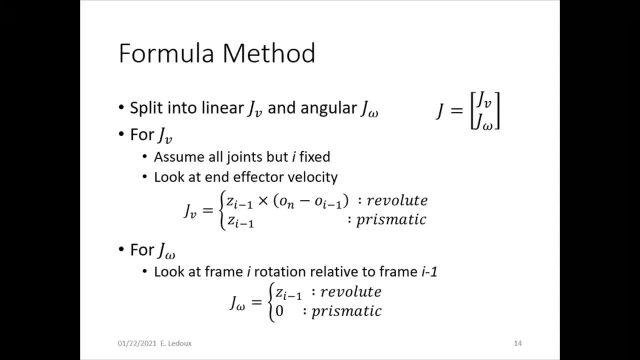 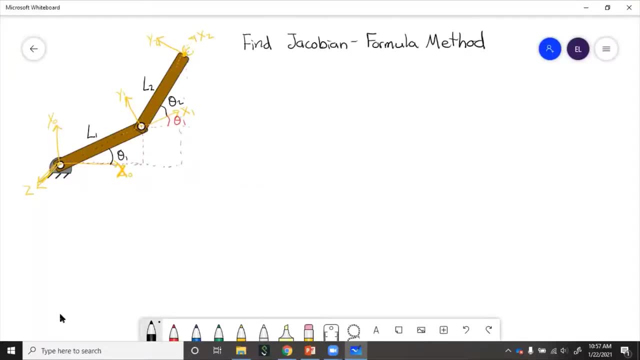 So now let's look at an example of how to calculate this. We need to find the Jacobian for this two-link robot using the formula method. Step one is find all of the joint origins, and all of these are in the zero frame. Step two is find the z-axis vectors. 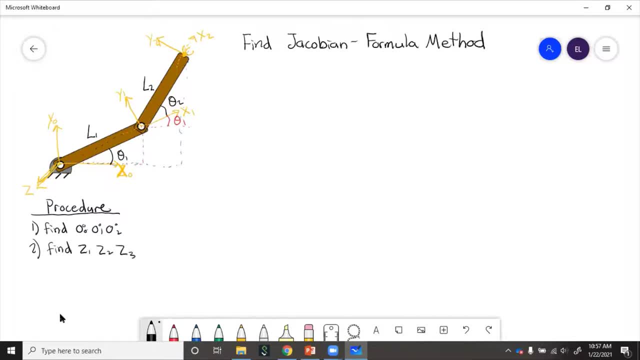 also given relative to the zero frame. Step three is: use formulas. These are all revolute joints, So So first we will find the joint origins O0,, O1, and O2.. O0 in the zero frame is just zeros. 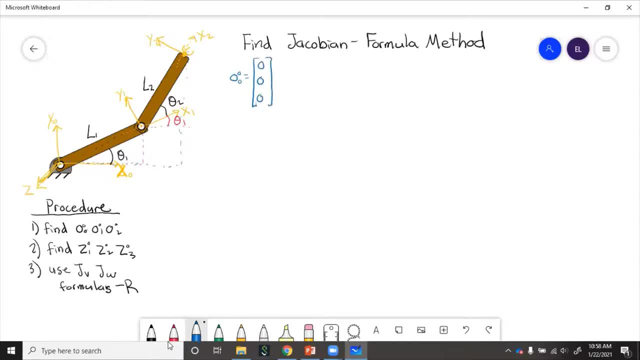 Then O2,, O1,. that's going to be this point. so that is L1, and then times cosine and sine of theta 1.. The final point is L1.. The final point is L1, and then times cosine and sine of theta 1.. 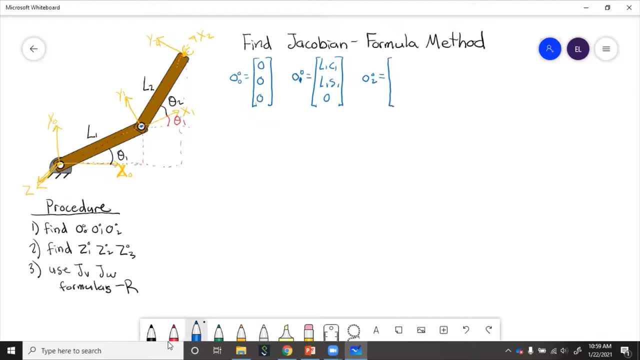 The final origin is going to be L2, added to origin 1.. Next we need to find the z-axis vectors. These are actually all the same. They all point out of the page. Then next, we need to use the formulas to get Jv and Jω, since these are revolute joints.